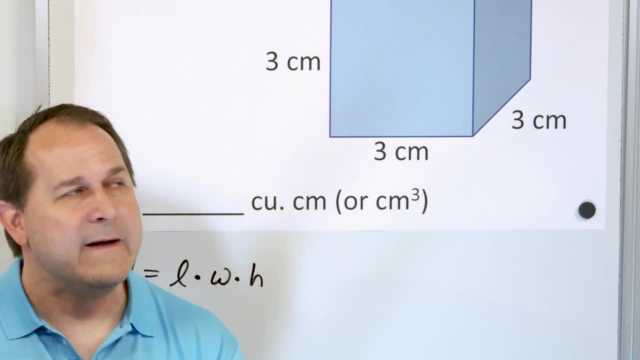 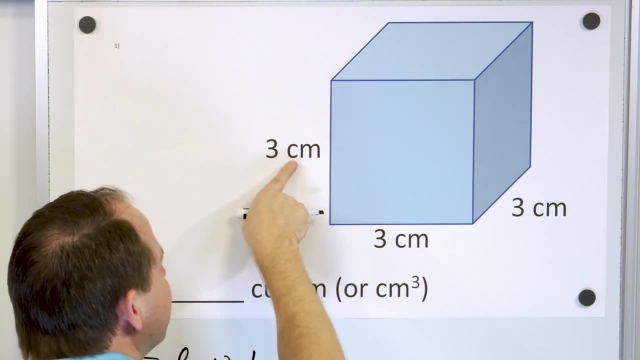 the surface area of a rectangle is just its length times its width. So if we were just trying to find the area of this square, we would be able to find the area of the square, which is the length of the square. forget about the fact that it's a cube: just the square here. we would just multiply length. 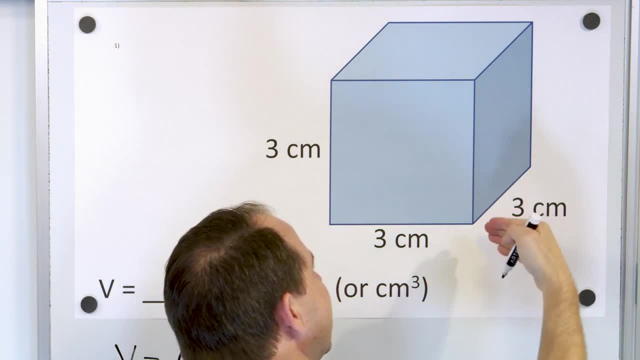 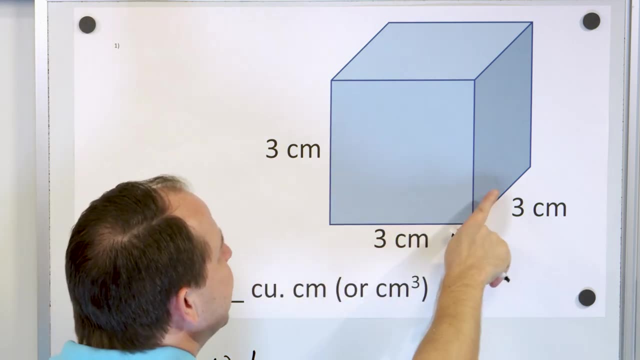 times width, three times three, right, But because it has another dimension to it, into the board, like that, also of a length of three, then to find the volume of the thing, it's three times three, but times the other three. So length times width, times height. Now, before we actually calculate it, 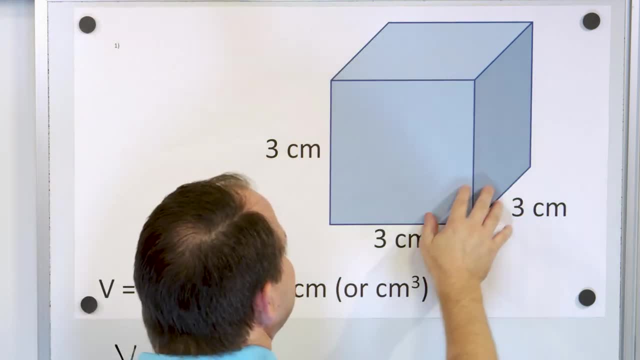 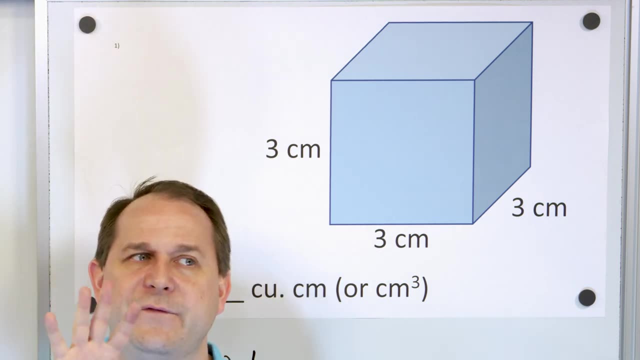 let's spend a minute to take a look. If we were to slice this thing up- remember what the area is- is trying to draw little squares onto the square. So if we were to slice this thing up, we would want to take a look at the surface to figure out how many squares fit in there. That's why the unit 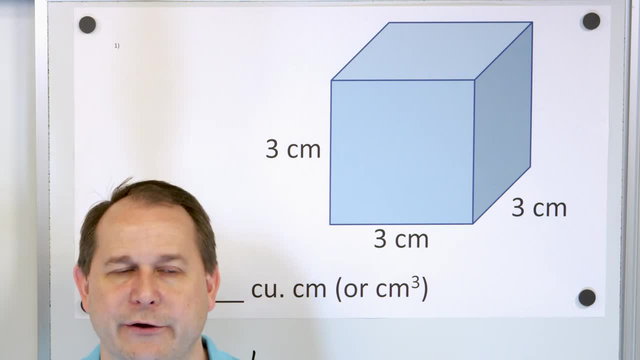 of area is square millimeters, square kilometers, square inches, things like that, But the volume. you have an object in three-dimensional space like this cube here, So we don't want to know how much the surface area is, We want to know how big the thing is in three-dimensional space. 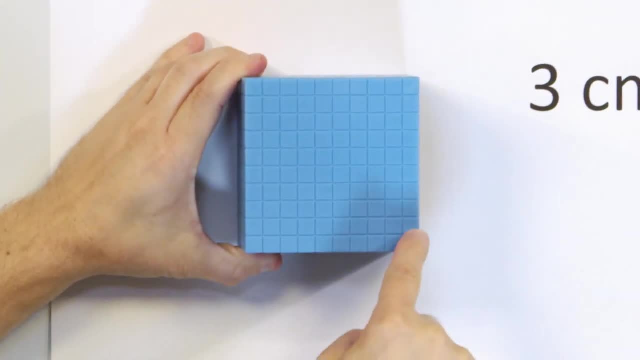 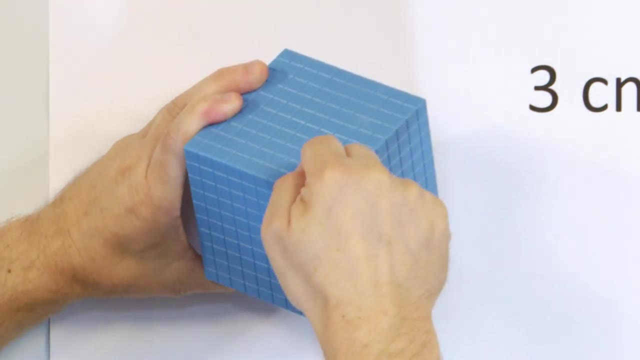 So if you see, if you look closely, this thing has a bunch of little cubes that are kind of cut into the surface, And if I turn it on its side, you can see that you could, if you wanted to, you could count these cubes all the way through, not just on the surface, but you could. 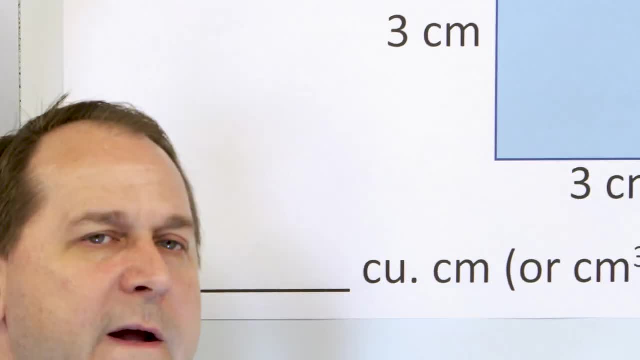 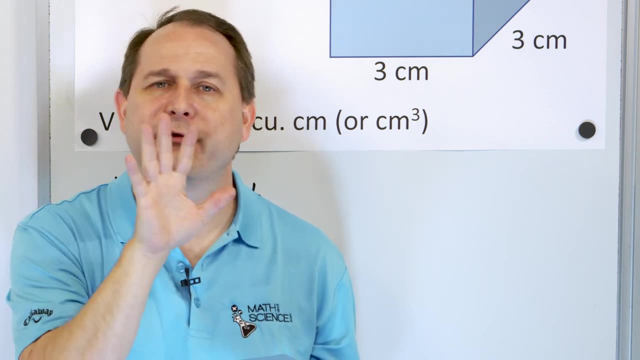 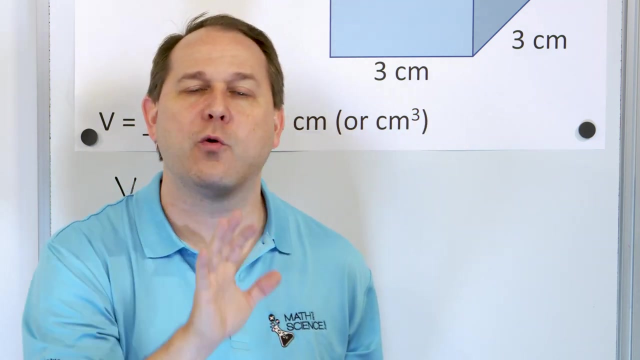 count the cubes on the inside all the way through, And so the volume of an object is trying to figure out how many of these little cubes fit inside. Just like for surface area, it's how many of those squares fit inside. So the units were square millimeters, square inches, square yards square. 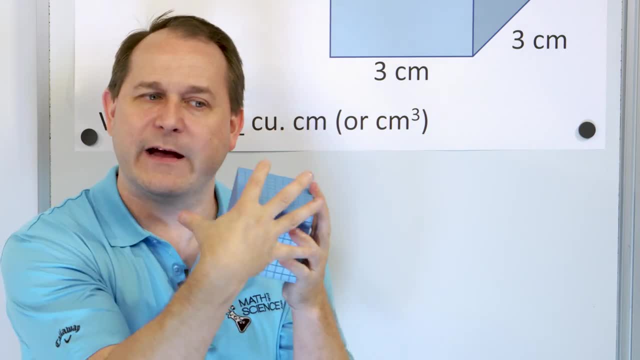 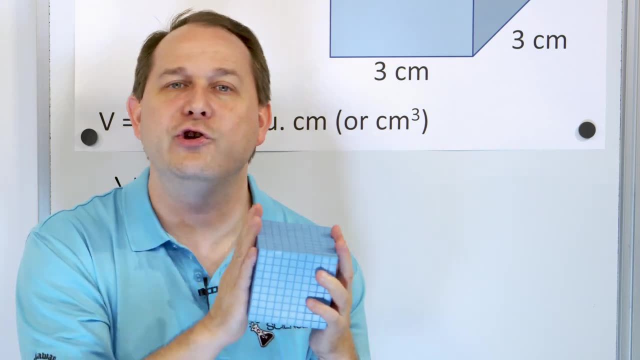 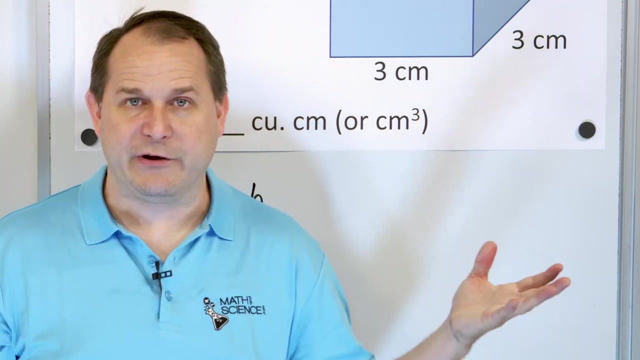 meters. But here we have a three-dimensional shape that takes up volume. So we want to figure out how many cubes occupy that volume. So the units will be cubic inches, cubic centimeters, cubic kilometers, cubic light years, cubic yards and so on. So the big picture here, when you're measuring just regular old. 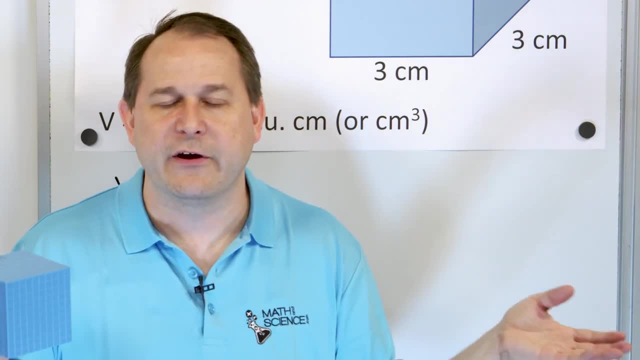 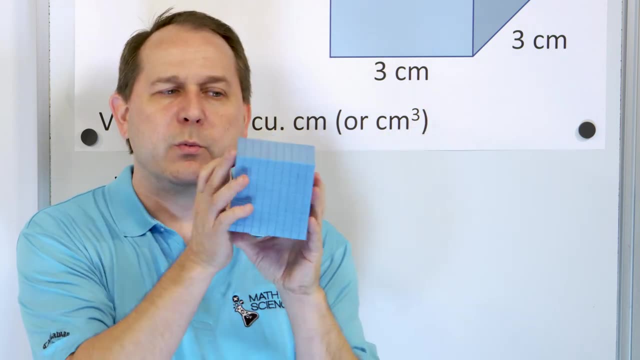 distance, the units are length like meters, kilometers, centimeters. When we're talking about area, we're drawing little squares and counting them: Square millimeters, square centimeters, square yards. When we're trying to find the volume, we want to see how much space. 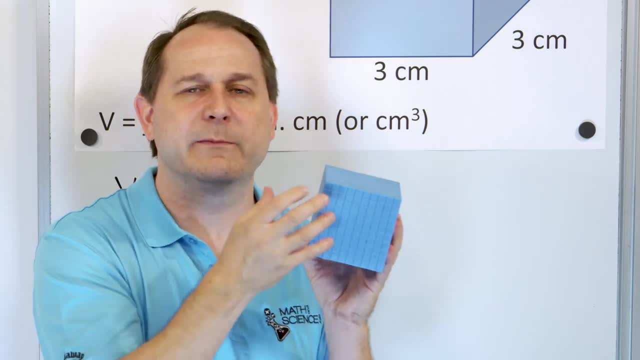 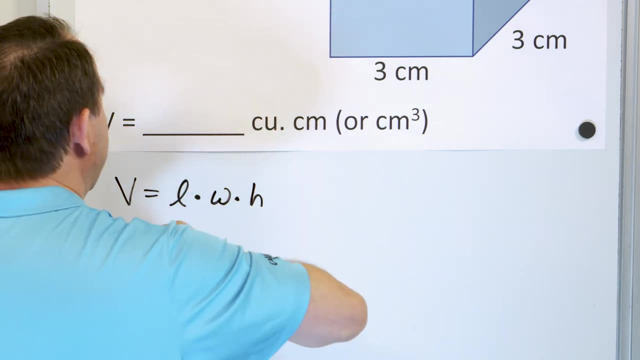 it occupies. We count cubes, So the units are cubic inches, cubic millimeters, cubic centimeters and so on. And so to then find the volume of this object we just said, length times, width times, height, it will be, in this case they're all three. So three times three times three. 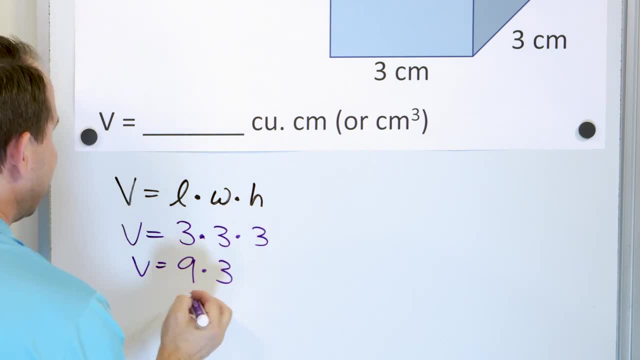 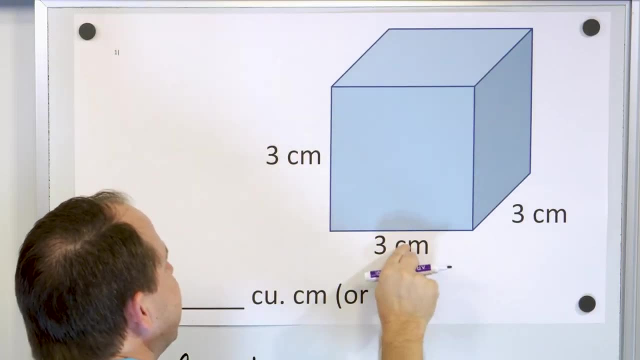 And so the first three times three gives you nine. Still have to multiply by that last three. Nine times three is 27.. Now, what units are we going to have? See for surface area. forget about this. It was just centimeters times centimeters. That's why we came up with the idea. 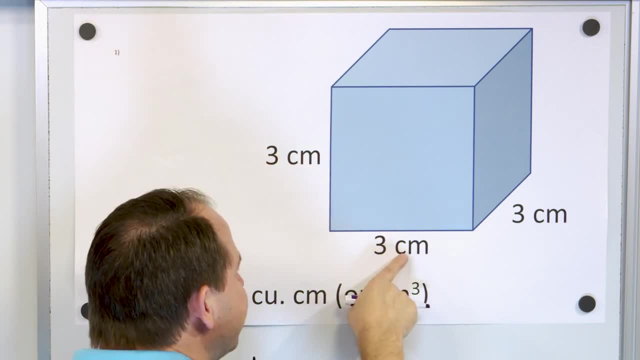 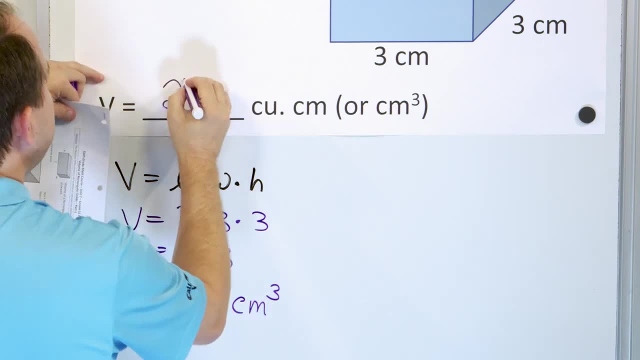 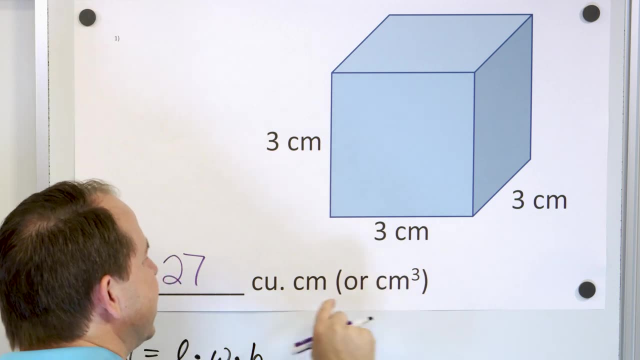 write centimeters cubed, So the answer is 27.. And we can say it out loud as cubic centimeters. That's what this means. Or we could say centimeters cubed. Usually we write it like this in science And the reason we have that little three up there at the top is just reminding you that it's volume. 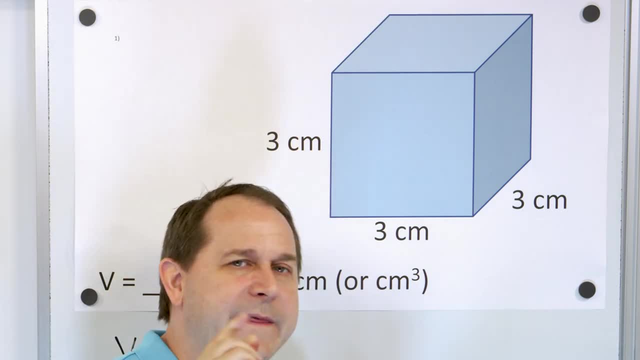 because it was one dimension of length and one dimension of width and one dimension of height and they were all multiplied together. So what we are having to deal with there is a unit of centimeters times centimeters, times centimeters, which means centimeters cubed, And so just to 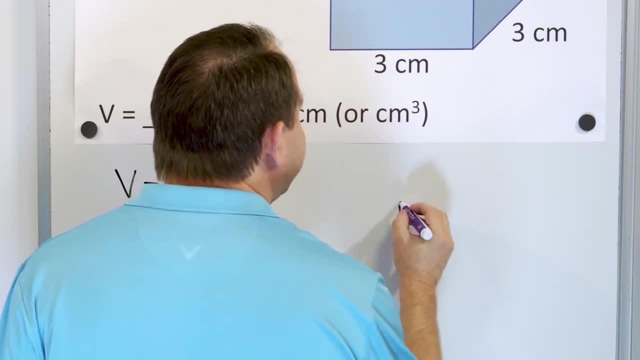 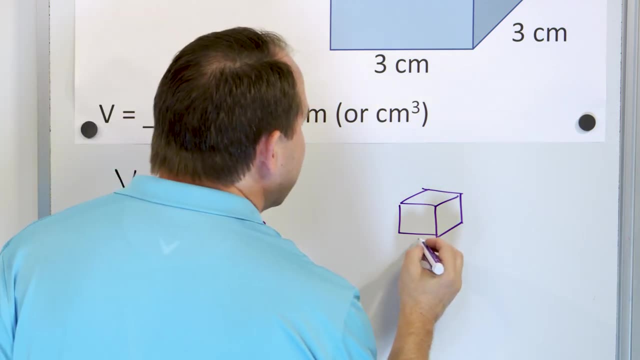 drill it home a little bit more. what we are really doing is we're trying to figure out how many- not squares, how many cubes will fit in there, where each of these little cubes in there has a one dimension of one centimeter and then the other dimension of another centimeter. 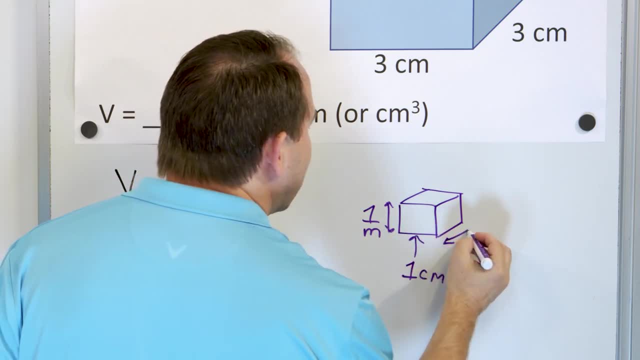 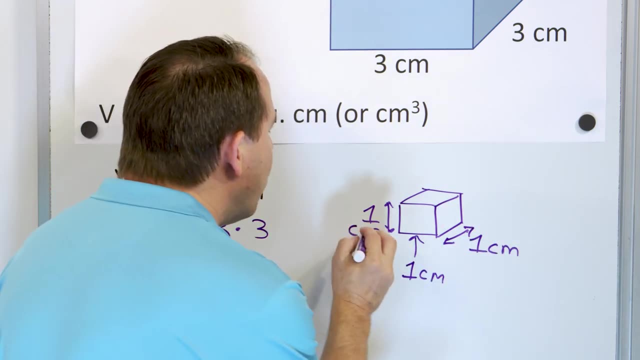 this dimension right here, and then the depth dimension, which is a little hard to draw on the board, another centimeter. So when we do that we're trying to figure out how many cubes will fit in there. When we say cubic centimeters we literally are saying: make a cube, where each of the distances 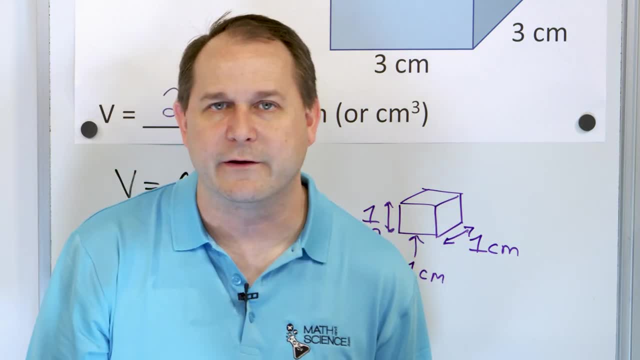 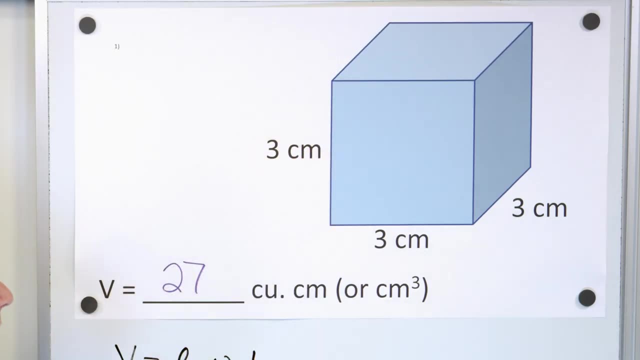 of that cube are just one centimeter. We call it a cubic centimeter. How many of these cubic centimeters can fit in there? That's what we're doing, And we're saying that 27 of these cubic centimeters can fit in there. So let's try to squeeze as much understanding as we can out of. 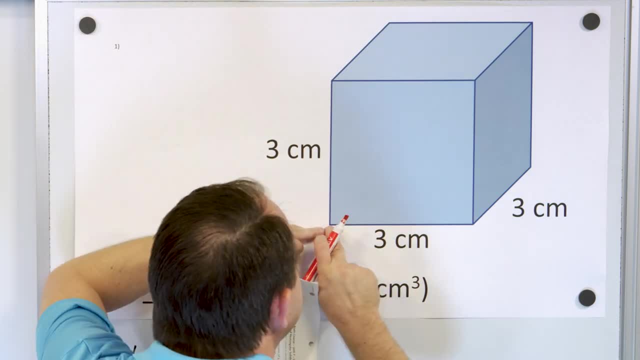 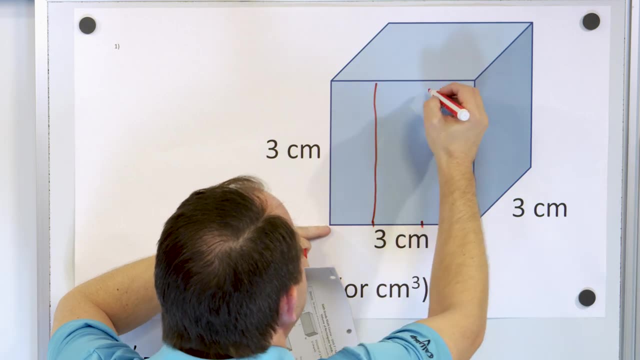 this by doing a little bit more. We know that if this is three, and if this is three then I could, if I were just trying to find the surface area, I could draw a little grid on top of here, and it's not going to be perfect because I'm not, you know, an artist and also my 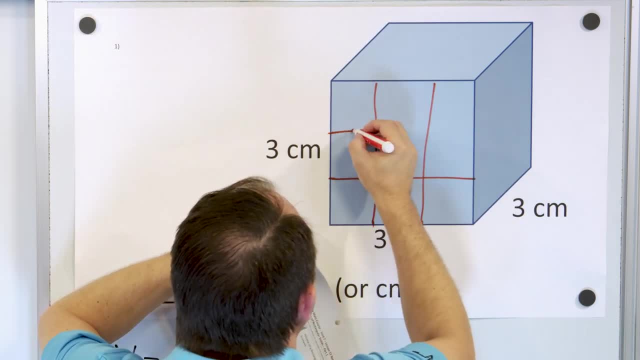 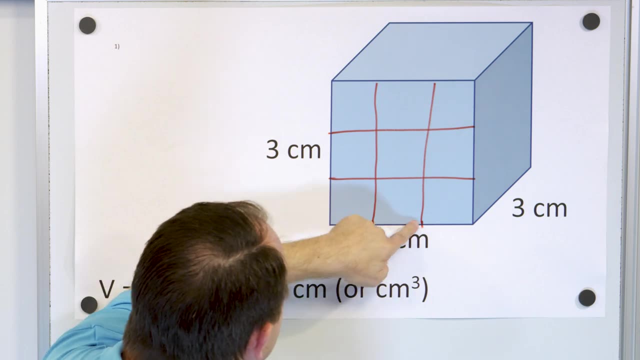 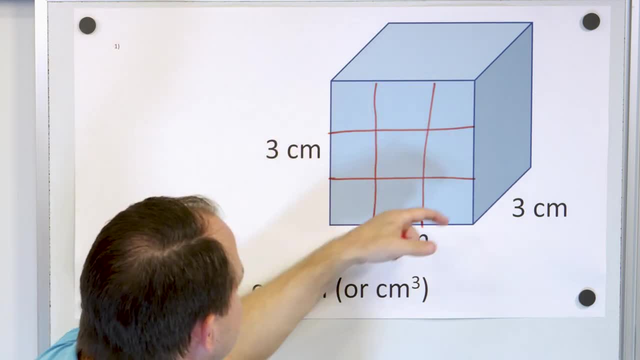 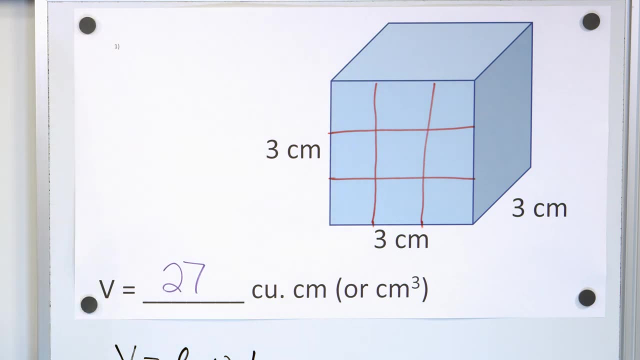 the area of the face here is three times three is nine square centimeters. You can count them: one, two, three, four, five, six, seven, eight. nine square centimeters fit on the face of this thing, Like counting the squares, just on the face of this right here, right, But we're not interested for. 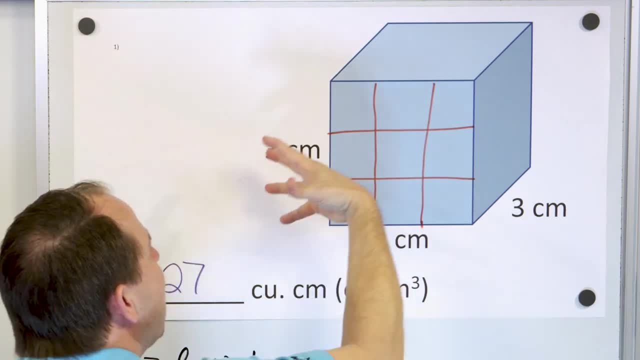 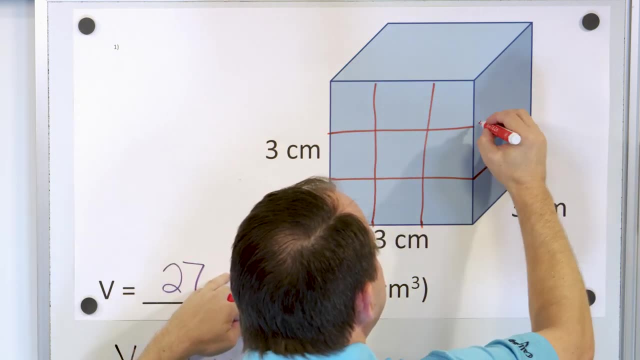 volume of just knowing how big the surface is. We want to know how big the entire space is. So then, if we know that there's nine of these squares on the surface, and then we can see that if we kind of go back here like this and we can- oh man, it's going to be a little hard. I'll draw it like: 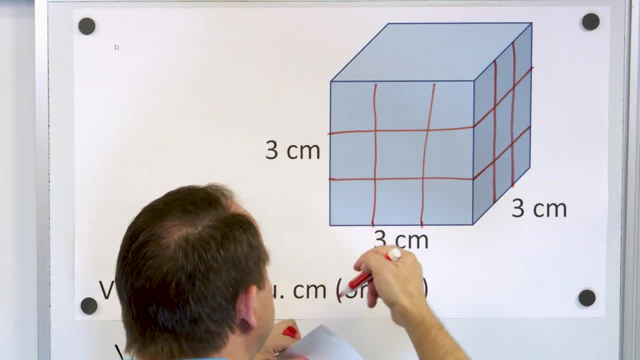 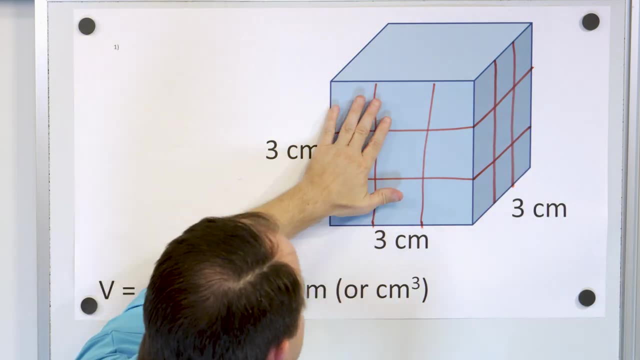 this. I guess If you could see, if you could cut it, because you know it's three centimeters in that direction also one, two, three, then you could see that there's basically going to be nine squares in this surface layer And then there's going to be nine more squares in the 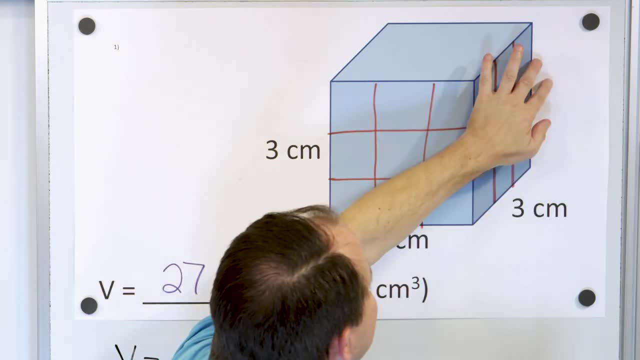 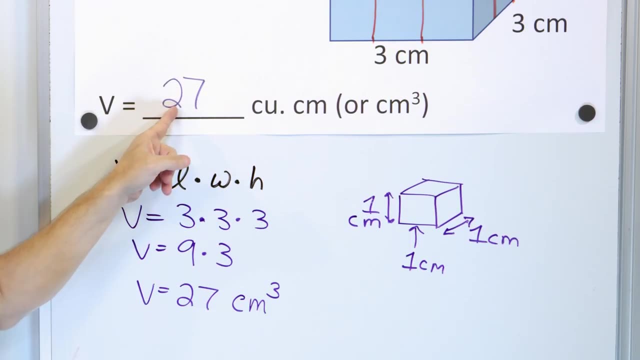 middle layer going through, And then there's going to be nine more squares in the last layer on the back end. So it's nine and nine and nine. that's nine times three, that's 27.. That's why there's 27 cubes, because there's nine of them in the first layer and then nine more in the second. 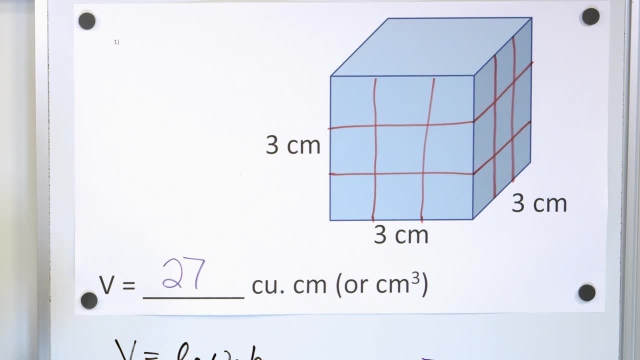 layer and then nine more in that third layer. So if we were counting we would get an answer of 27 cubic centimeters. Same thing I was saying down here. we just figure out how many of these are in here and we count them For a rectangular solid like that it's. 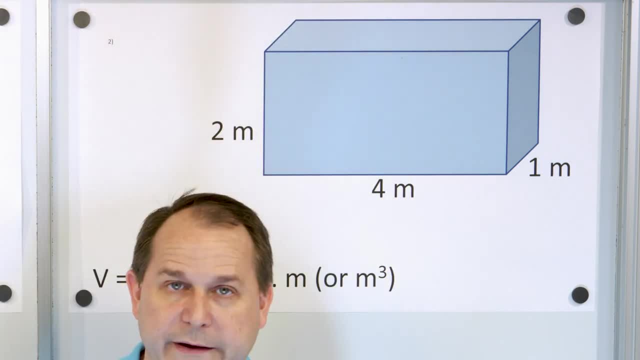 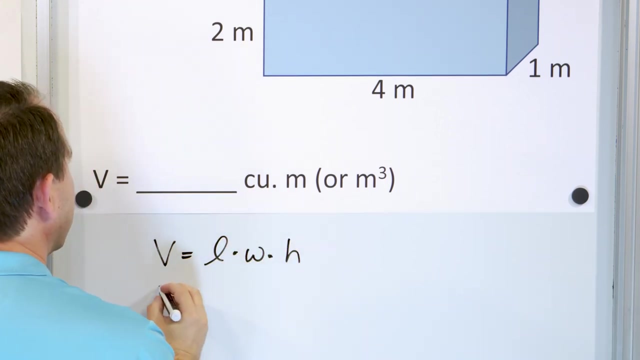 always length times width times, height, always, And that is what we have to remember. So now that we've done the talking, we can calculate much more easily this: We're going to find the volume of this thing And it's length times the width times the height, always four rectangular solids: The length. 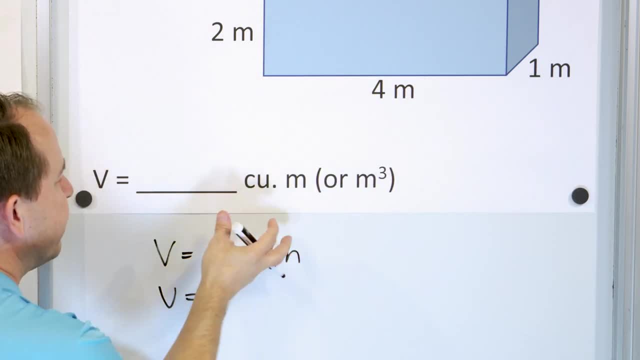 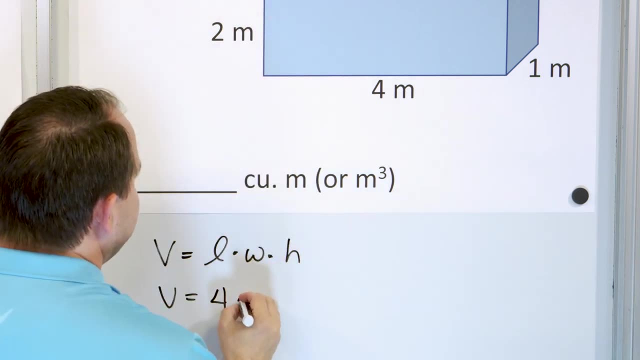 times the width, always four. And these numbers don't really matter which place you put them, because you're just multiplying them. They're all going to give you the same answer, no matter the order in which you multiply. So four goes here, two, let's say there, And I guess two is really. 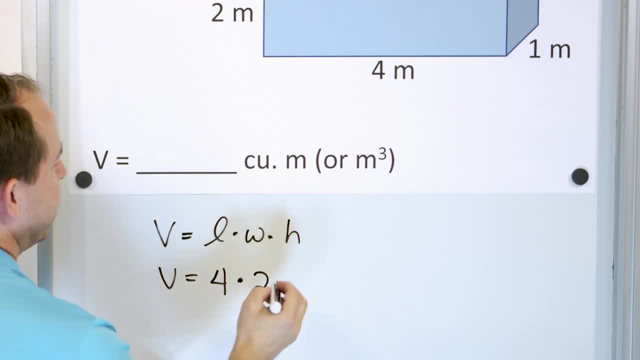 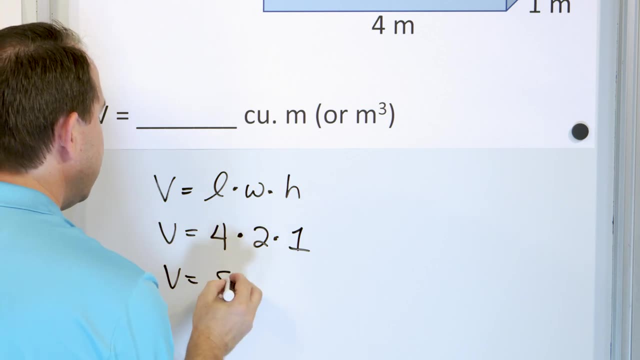 the height and the depth is really. it doesn't really, I can say, matter what number you put where, because you're multiplying them anyway. So four times two times one is the same as two times four times one, for instance. So you have eight times one, which is still a volume of eight, And it is meters times meters. 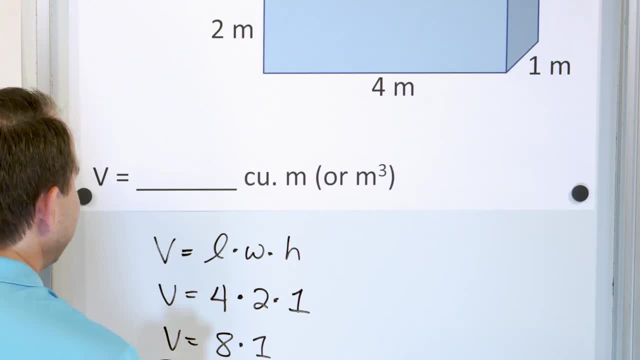 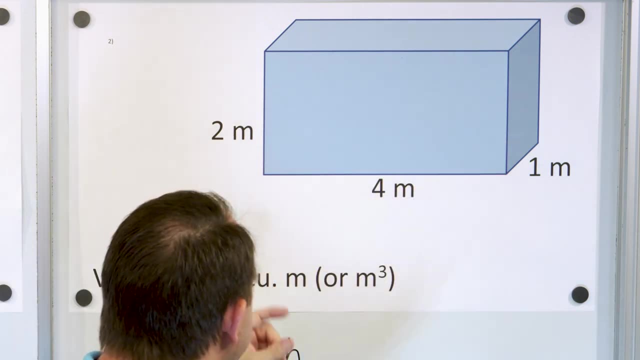 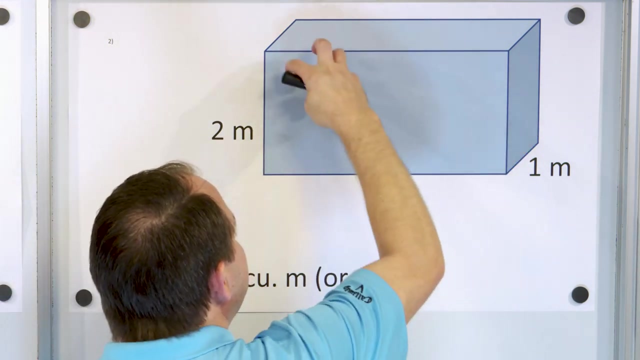 times meters, which means cubic meters. So the answer is eight cubic meters. Now what this means is, if I actually built a cube of these dimensions, then if I took a little cube that was one meter on each side, also called a cubic meter, and try to see how many of these would fit in there, then eight of them would fit in. 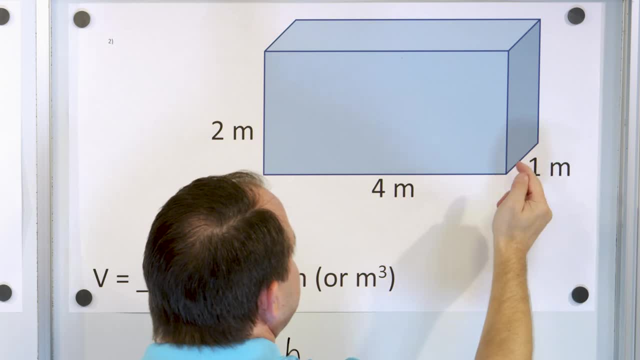 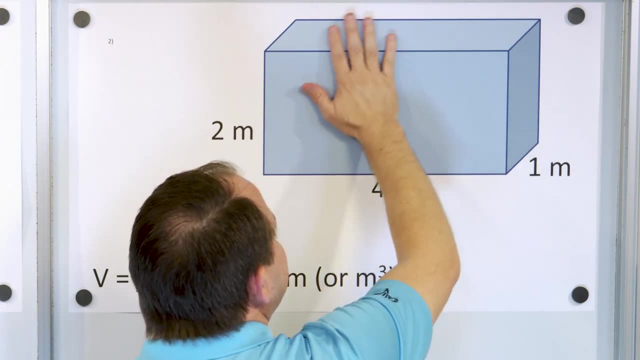 there, Because on the surface layer here, well, actually it's only one meter deep. you can see that there would be two times four, there would be eight squares here and the depth is only one. So there's only eight of these cubic meters that will fit in there in that space. 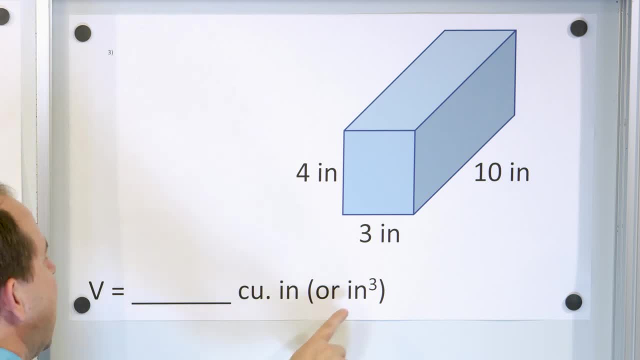 Right Half of the battle is understanding why the unit of volume has a three there. It's just because you have the third dimension And it's telling us that you know meters times meters, times meters cubic meters. that's what the meters cube. 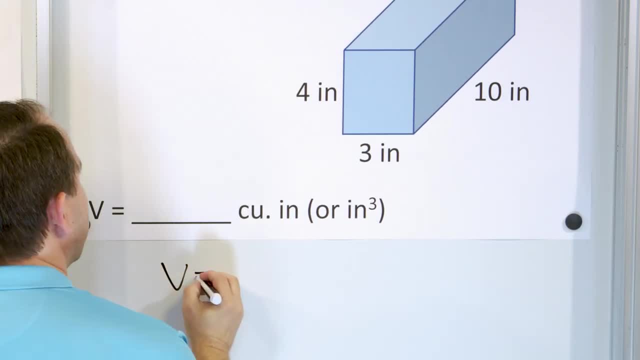 means how many of those will fit in there? What is the volume of this guy? It is length times width times height. Right Again, it doesn't matter what number you put in what position, because it's all going to be the same anyway. So I'm not going to stress out about which one is which One of. 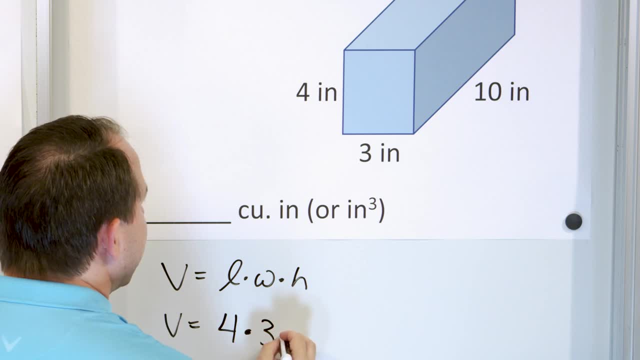 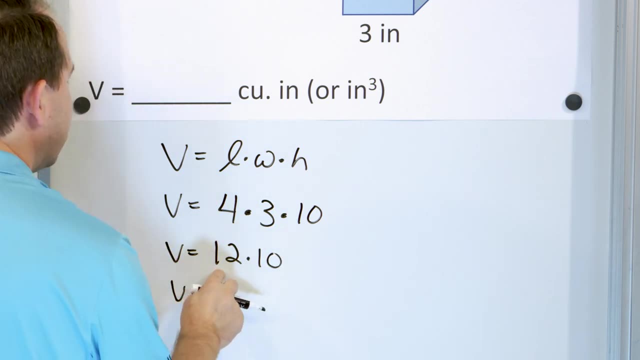 them has to be a four, the other one has to be the three and the other one has to be the 10.. We're multiplying them all anyway. Four times three is 12, we still have to multiply by 10.. And 12 times 10, you just add a zero and make it 120.. 120, what? 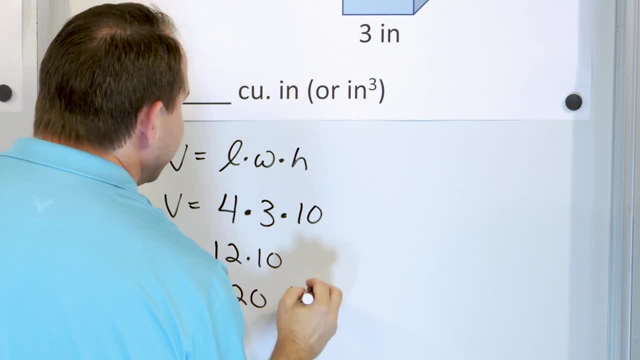 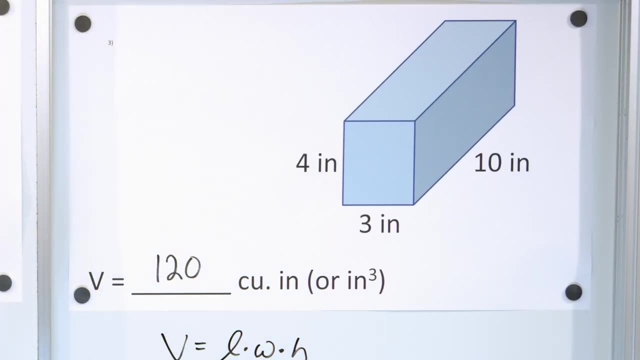 Well, it's inches, times inches, times inches, which means it's cubic inches. That's how many cubic inches will fit inside of here? 120 cubic inches. I do have a couple more. I'm going to take these down and conquer those right now. 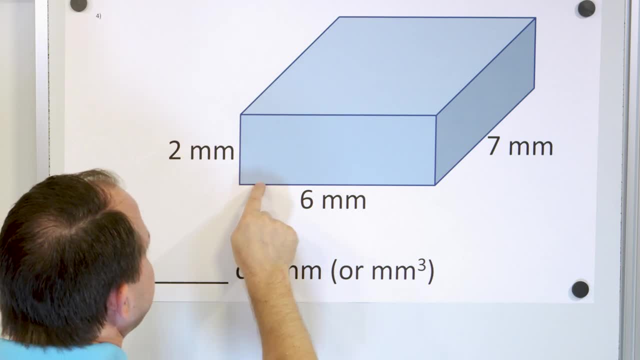 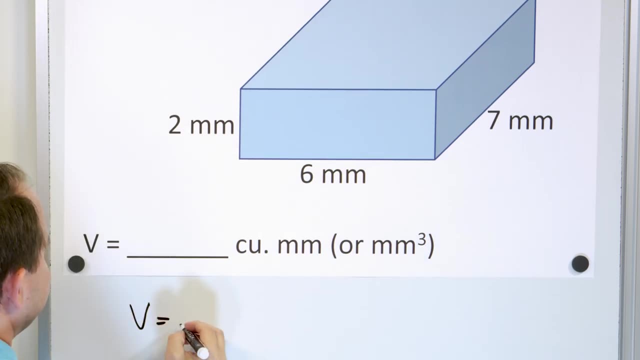 Alright, the next problem. we have this rectangular solid. we have one dimension of six millimeters. The height here is two millimeters, the depth here is seven millimeters. The volume is always the same. It's the length times the width times the. 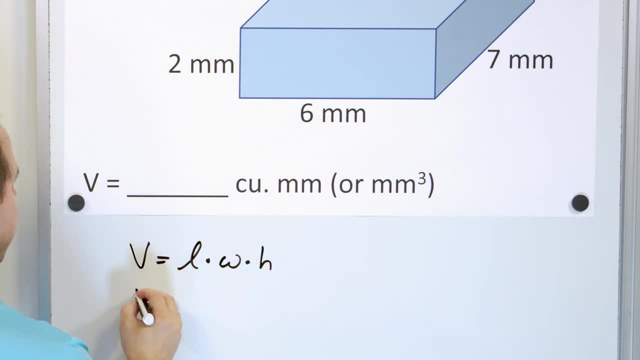 height, or length, width, depth, however you want to talk about it, the length of this thing, and you can call each dimension. you know which one's length, which one's width. I mean, it doesn't really matter. The length I'm going to say is six. 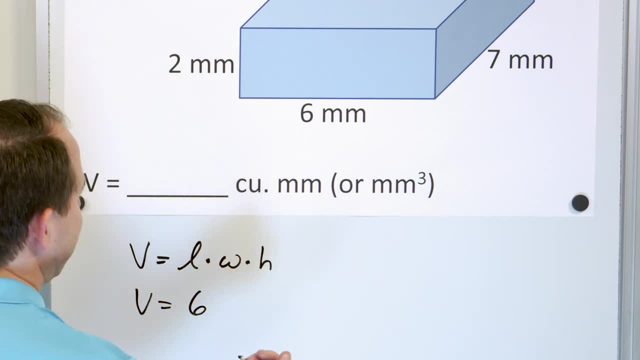 even though really most people would call that the width. You see what I'm saying. It doesn't really matter. right. 2 for the other dimension, even though most people would call that height. I'll just put it there. 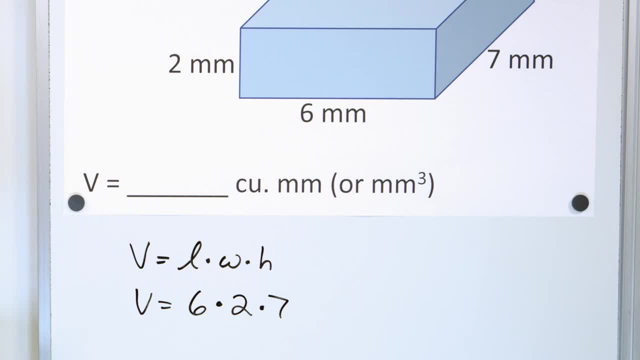 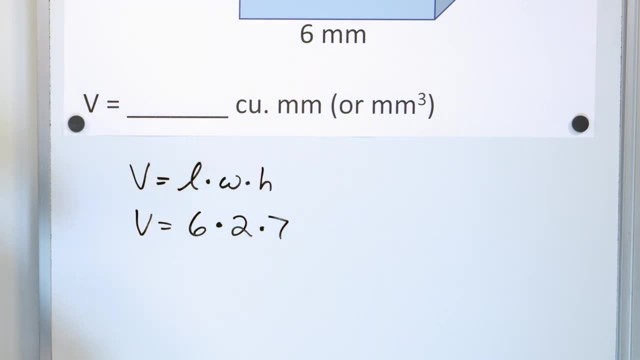 It doesn't really matter. And then 7 for the depth. all right, So most people would probably call this length, This would be width, This would be height. So the numbers would be rearranged, But the answer will be the same. 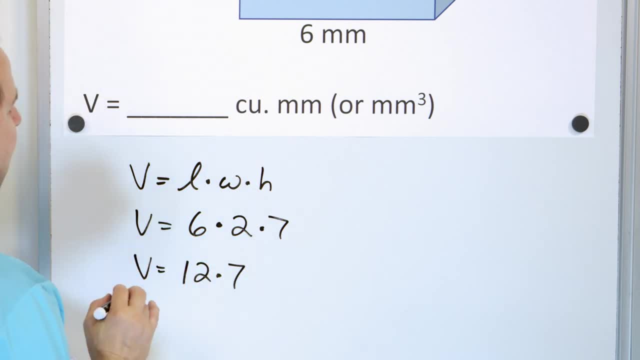 So 6 times 2 is 12.. Still got to multiply by 7. And 12 times 7 from multiplication tables is 84. And you can multiply that out by hand. if you needed to 84, what Millimeters times millimeters times millimeters? 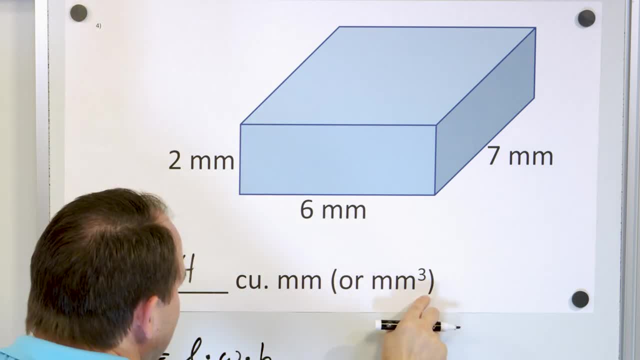 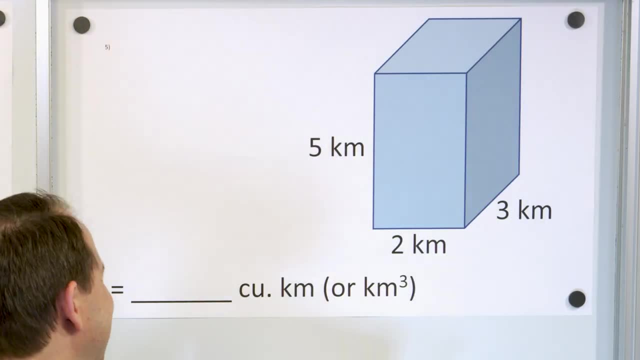 means that the answer is 84 cubic millimeters, or also called millimeters cubed there. all right, 84.. All right. now here is our very last problem. We have more of a skyscraper shape here. The volume is still a rectangular prism. 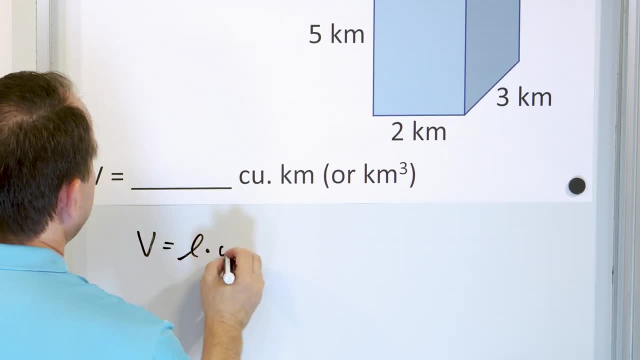 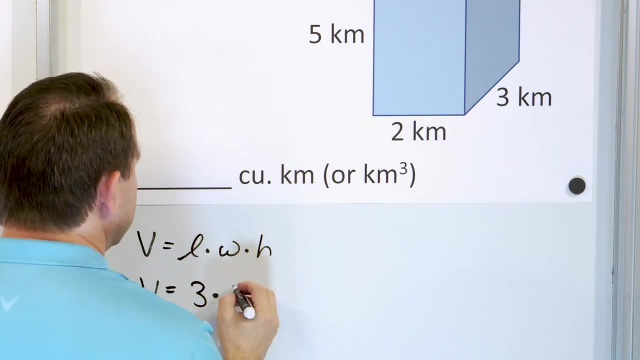 So we have a rectangular, solid: Length times width times height. right, We could say that the length is 3.. The width is 2, and the height is 5.. Again, I don't care where you put the numbers, because you're just gonna have to multiply them. 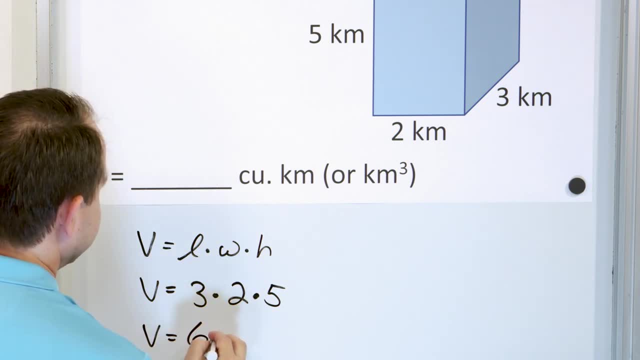 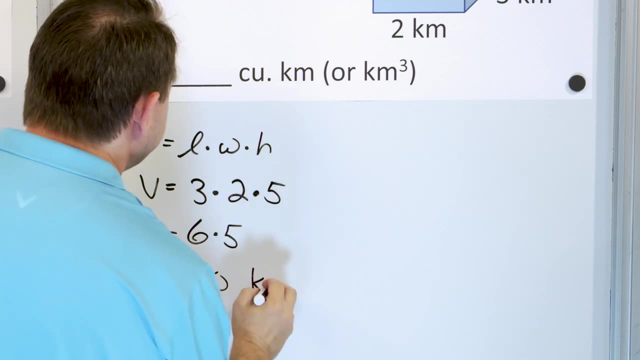 all together anyway, The volume 3 times 2 is 6.. Still have to multiply by 5.. 6 times 5 is 30.. And the units are kilometers times kilometers times kilometers, which means kilometers cubed, And there's 30 of them. 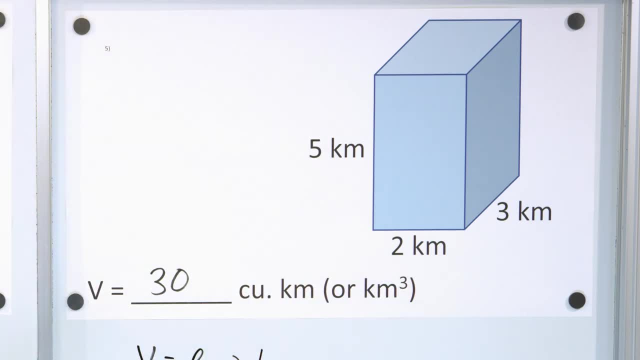 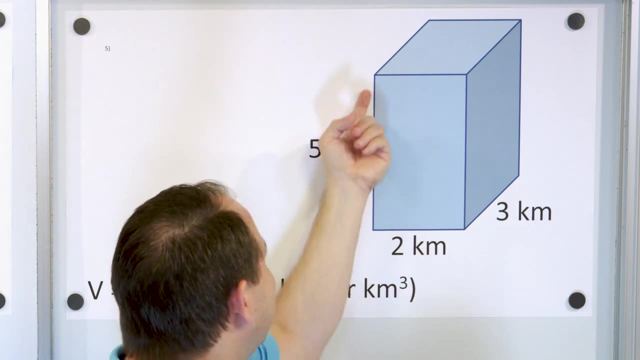 30 cubic kilometers, or 30 kilometers cubed. So what this means is, if I actually built a skyscraper where the width of it was this much and the depth was this much and the height was this much, then I would be able to fit 30 of these little cubes inside. 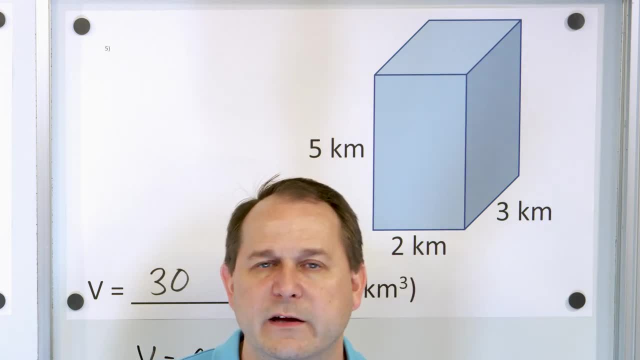 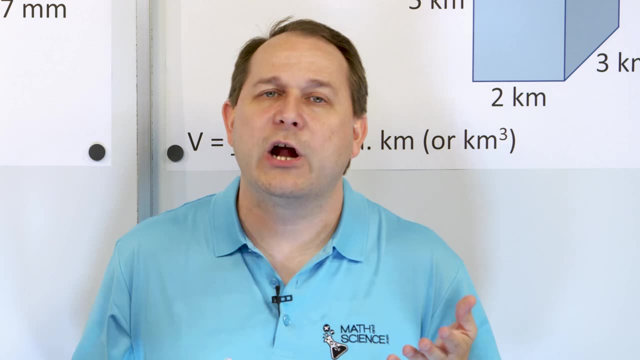 where each cube had a side and all directions of one kilometer. 30 of them. That's what would fit. So there's really two goals here. One, I want you to know how to calculate the volume, but two, I want you to understand.